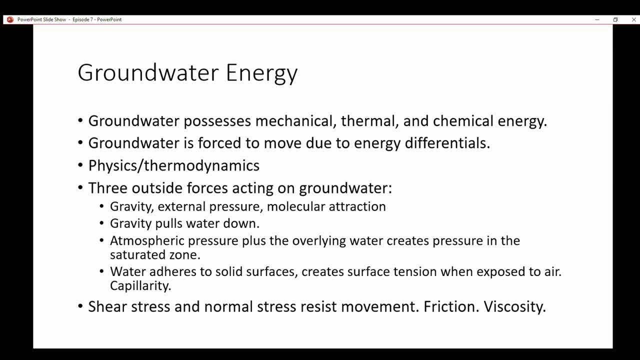 water adheres to solid surfaces, creates surface tension. when exposed to air such as we, such as the capillary fringe that we talked about a few episodes ago, capillarity And sheer stress and normal stress resist movement, which creates friction, which creates viscosity And viscosity. 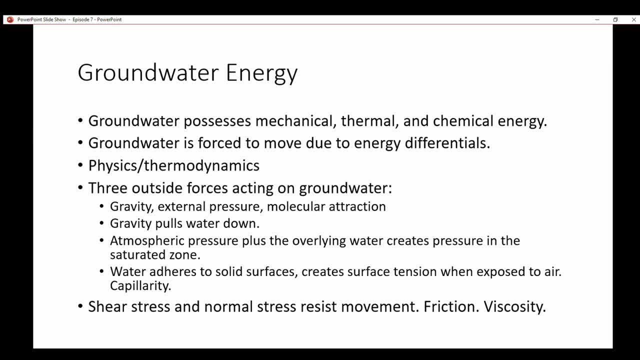 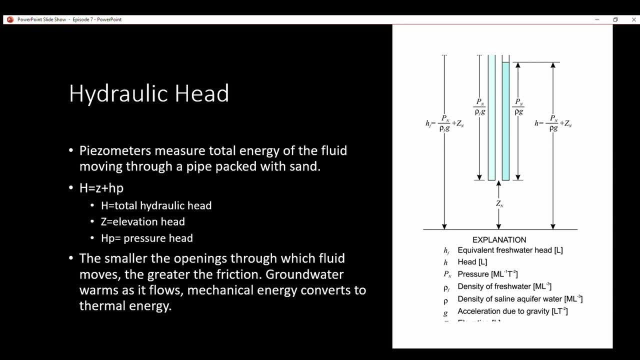 if you remember, is the resistance to flow of a fluid. So the hydraulic head piezometers which you can see on the right measure the total energy of the fluid moving through a pipe packed with with sand. And to figure out hydraulic head, you find the elevation head. you add it to. 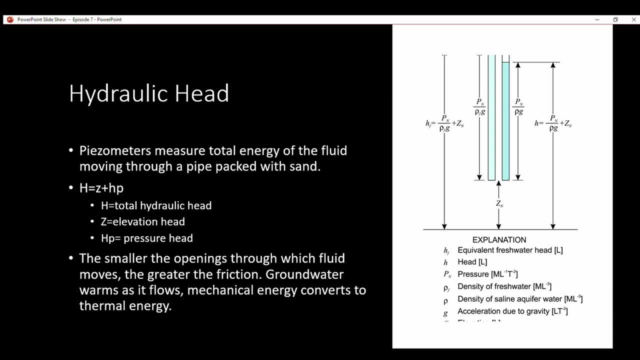 the pressure head. that'll give you your total hydraulic head, And the way I calculate it professionally is you take the elevation datum that you have from a surveyor, for instance, and you subtract the the, the level of, the level of. 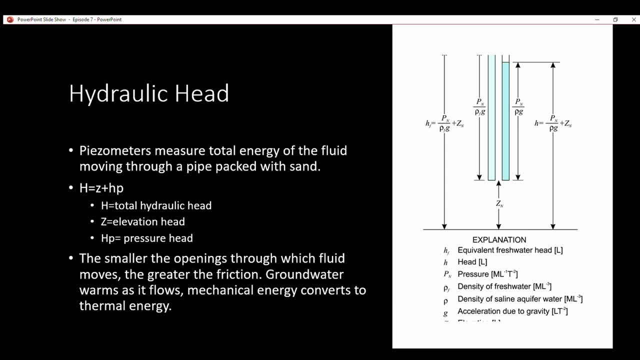 the level of groundwater, the the water table measurement. you subtract the elevation from that and that'll give you your hydraulic head as well. So the smaller the openings through which fluid moves, the greater the friction. Groundwater warms as it flows and mechanical energy that makes the water 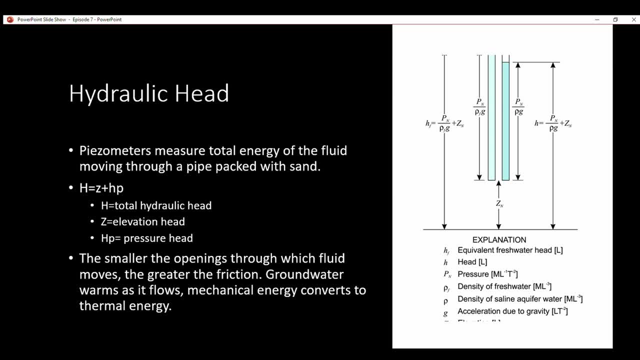 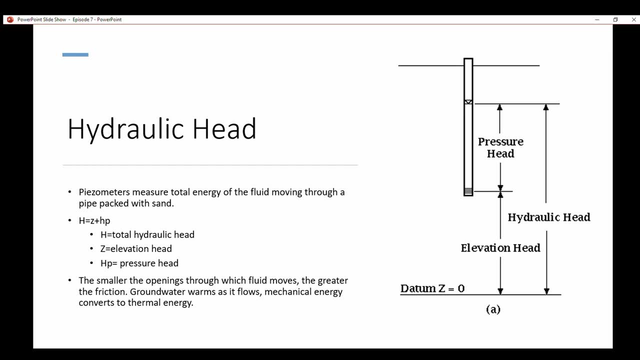 flow is converted to thermal energy. So, piezo, Oh, I uh, apparently I I uh doubled a slide, but this kind of shows you. uh, this is a better diagram of the hydraulic head. You got the pressure head, the elevation head added. 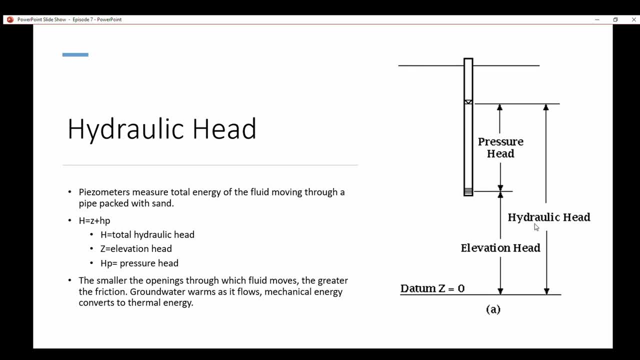 those two added together create your hydraulic head. And when you take your water level, obviously the triangle is the water table, and if you know the elevation of this PVC pipe, you can figure out hydraulic head that way too. So you can figure out hydraulic head that way too, by subtracting the elevation from the uh. 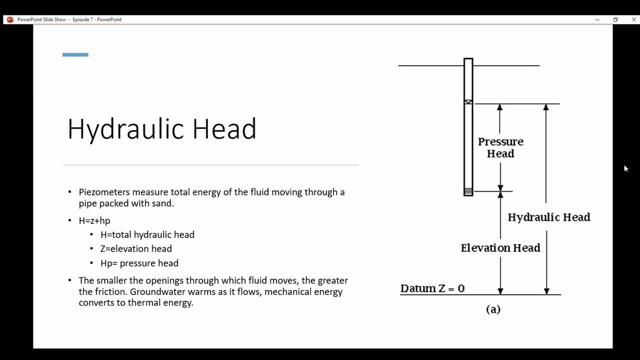 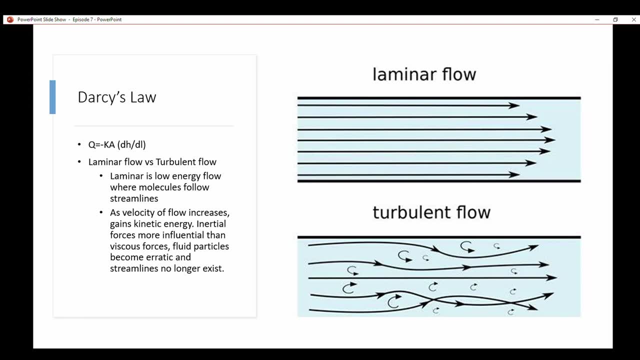 the hydraulic head, I mean the water table level measurement. So Darcy's Law- And this is review- in terms of the formula, Q, which is uh- the discharge, equals negative. K, which is uh- hydraulic conductivity. A is the cross-sectional. 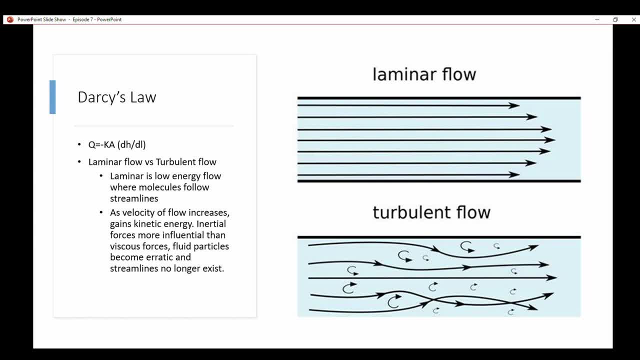 area DH over DL or hydraulic gradient, which is the change in head, over the change in length. And uh, you have laminar flow versus turbulent flow. So laminar is low-energy flow where molecules follow streamlines. 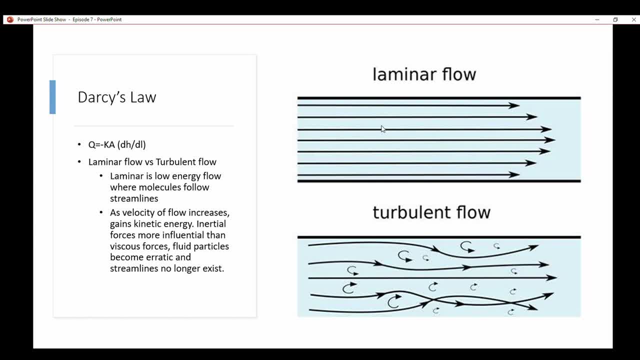 as you can see in this picture right here. And as the velocity of the flow increases, it gains kinetic energy, Inertial forces more influential than uh, the viscous forces. Uh, fluid particles become erratic and streamlines do not exist anymore, as you can see in this. 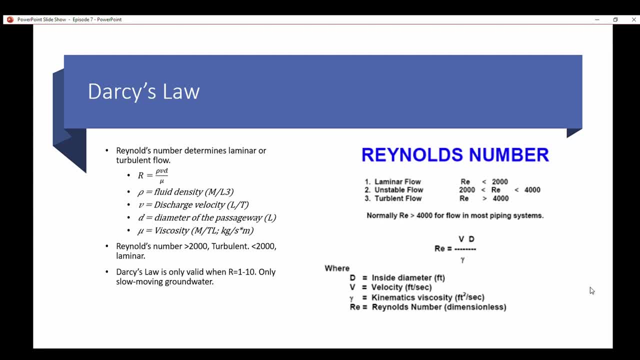 in this photo And there's a reason why we're talking about this. So the Reynolds number it- and this is kind of review. if you uh took sedimentology, you learn about Reynolds number. I think it's also in geotechnical textbooks as well. 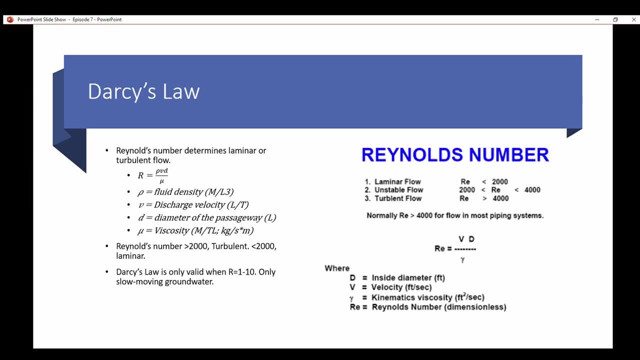 But the Reynolds number determines whether a flow is laminar or turbulent And the formula is: R equals fluid density times discharge velocity times the diameter of the passageway divided by the viscosity And fluid density is, in uh measurement, divided by length, cubed. 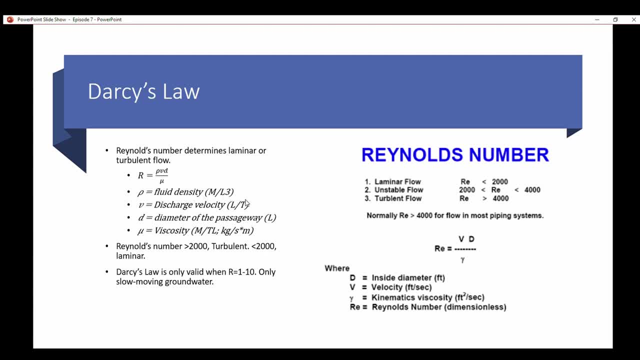 Length times time for discharge velocity, such as meters per second. Diameter of the passageway, so an inch or a millimeter. And then viscosity is uh a measurement divided by uh time times. length, So kilograms divided by the seconds times meters. 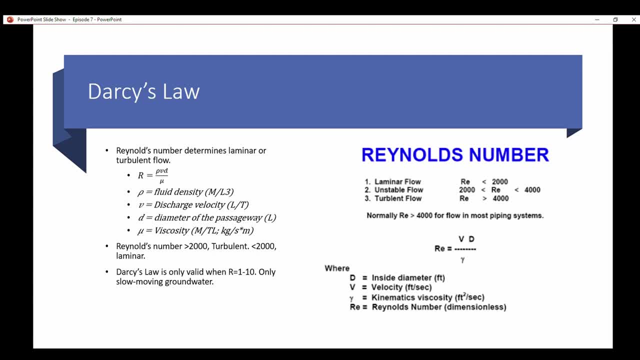 So if the Reynolds number is over 2000, it's turbulent, Um, and then if it's less than 2000, it's turbulent, If it's less than 2000, it's laminar. And well, actually it's valid when the Reynolds number is between 1 and 10, I guess technically. 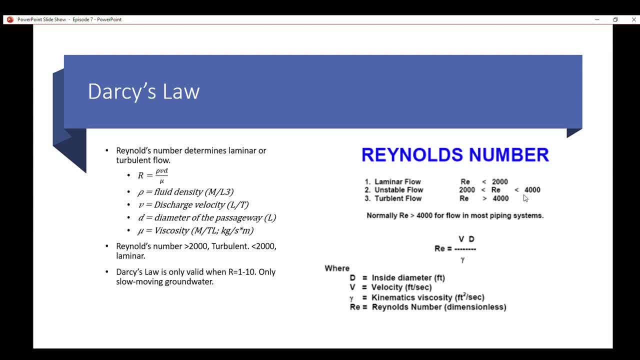 Because, uh, groundwater does not move that fast in the ground. Um, typically, when you're using Reynolds number, you're also talking about stream flows, which can be very high, very turbulent. Uh, in terms of water moving inside the ground, it's moving at very low rates. 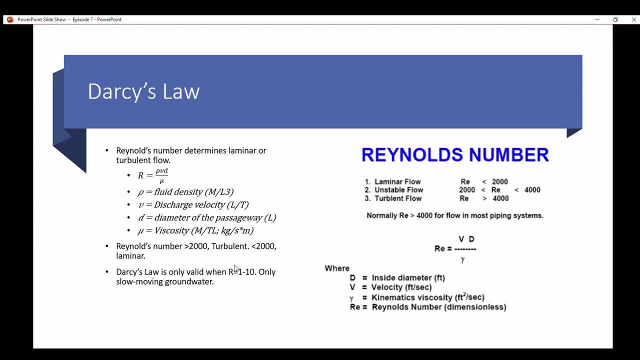 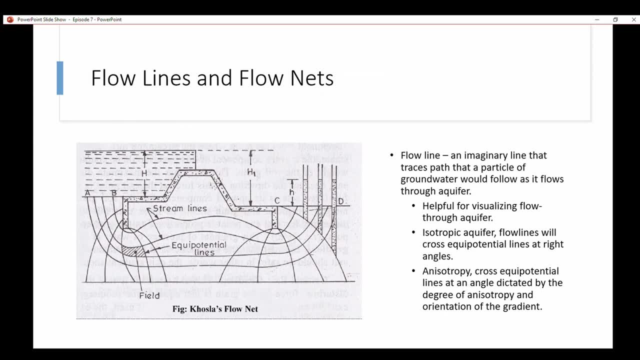 which is why, uh, Reynolds number between 1 and 10 makes Darcy's Law valid. So, uh, flow lines and flow nets, as you can see in this picture. Uh, a flow line is an imaginary line that traces the path of a particle of groundwater. 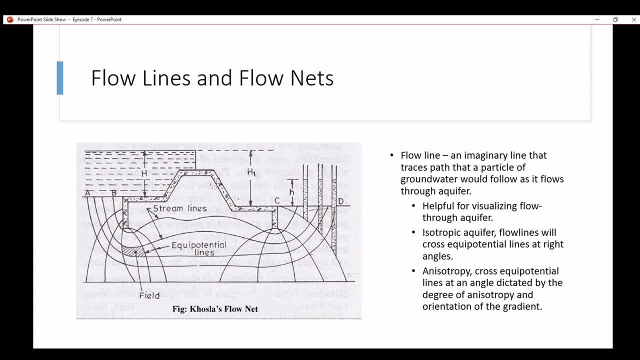 Uh, the path that a particle would flow uh would follow as it flows through an aquifer. It's helpful for visualizing flow through aquifer. An isotropic aquifer flow lines will cross equipotential lines and anisotropy. 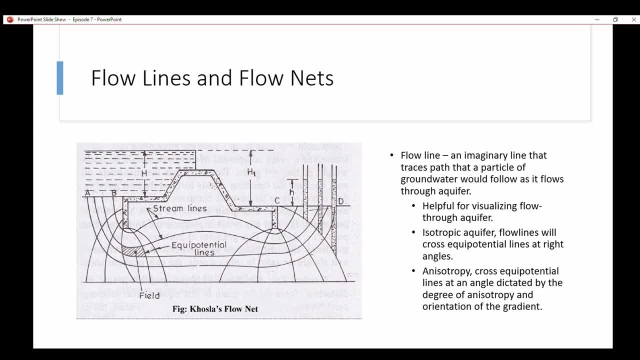 Uh, cross they. the equipotential lines will be crossed at an angle dictated by the degree of anisotropy and the orientation of the gradient, So this looks like it's isotropic. this aquifer Based on. based on this. 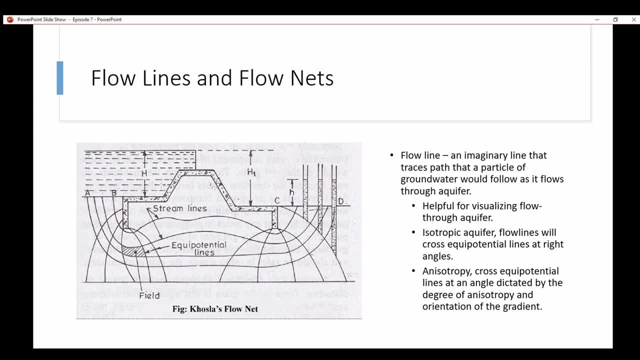 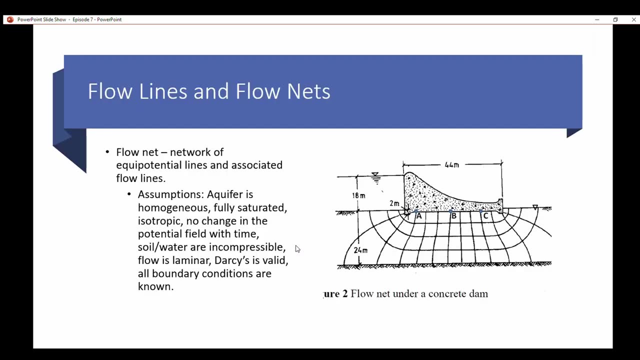 But if it's not perpendicular, the flow lines and the equipotential lines- they call it stream lines in this diagram, but they're not uh perpendicular. it's most likely because of anisotropy. So a flow net is basically the culmination of uh equipotential lines. 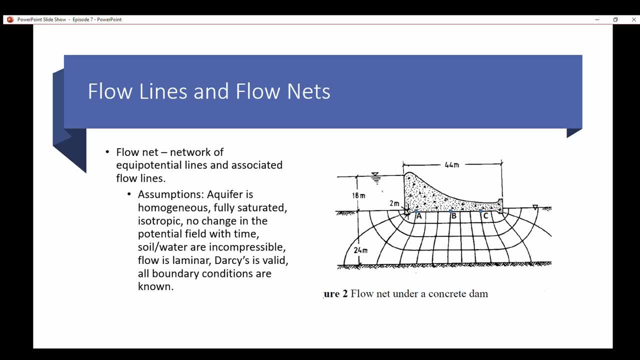 which are just groundwater contours, really, and the associated uh flow lines. There are assumptions made about this. There are assumptions made when doing a flow net. So you you assume that the aquifer is homogenous, it's fully saturated, it's isotropic. 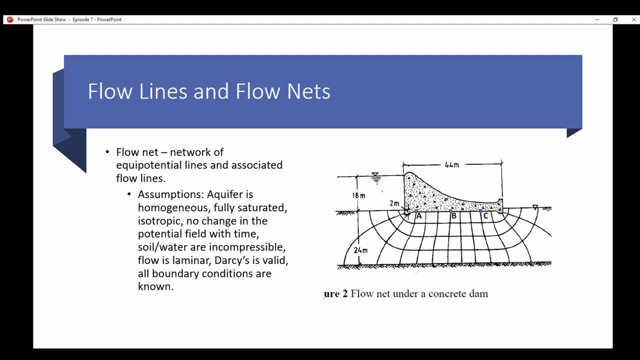 and these are review terms, but homogenous basically means the same material throughout. Isotropic means that uh groundwater flow is equal in all directions in terms of velocities, um in terms of permeability, as I should say, Um the vertical and uh horizontal hydraulic conductivities will be equal. 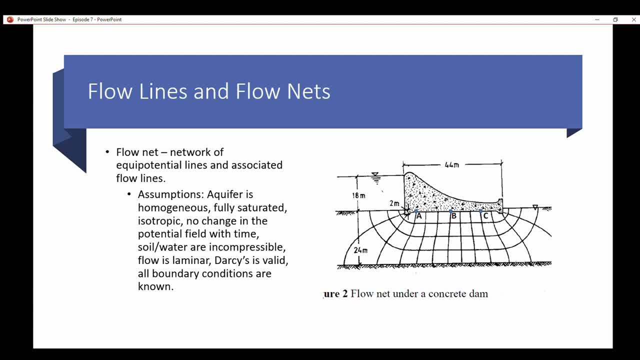 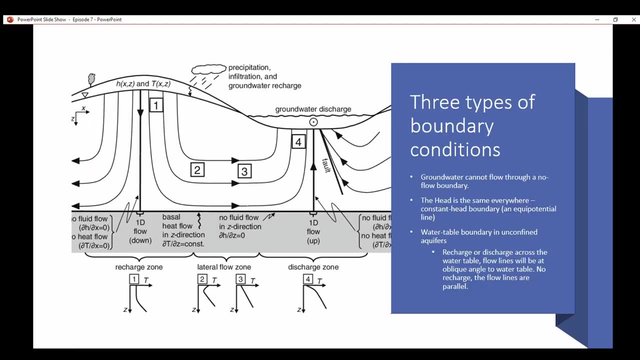 There's no change in the potential filled with time. Uh, soil and water are incompressible. The flow is laminar, and which makes Darcy's valid, And all boundary conditions are known, And there are three types of boundary conditions.